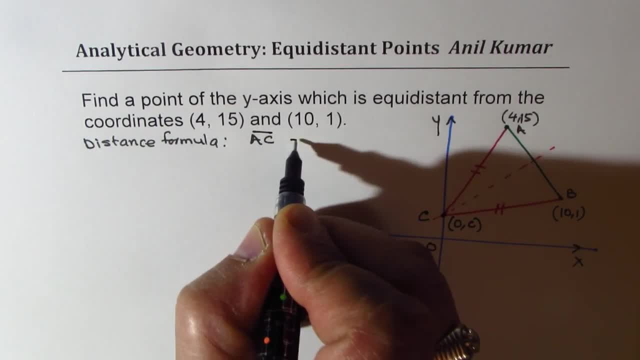 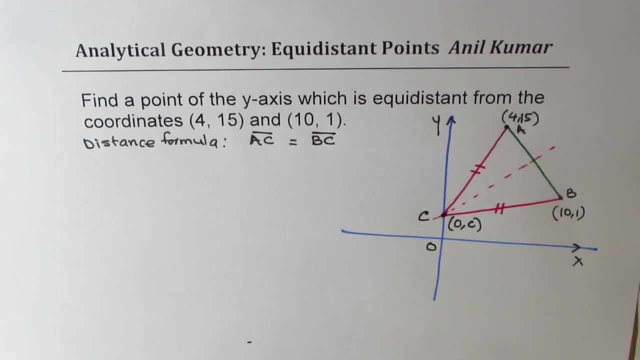 Since we know that length AC is equal to the length BC, So these two lengths are exactly same. Some of you may like to put like this right: Absolute value of these two lengths should be same. Now, if lengths are same, even their squares will be equal, correct? 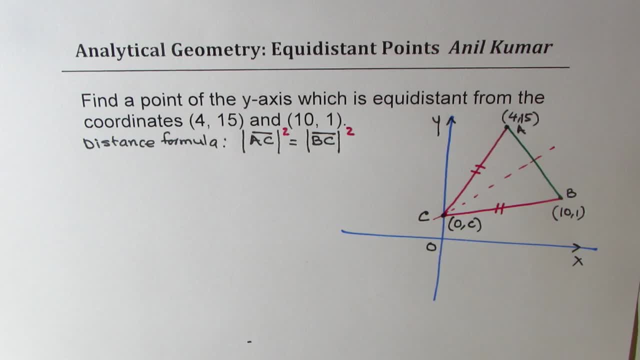 So we need not get into square root kind of things. Perfect. So I hope that gives you an idea of how to solve this particular equation. Now let's begin. So we are saying that AC is equal to BC. So we are saying that AC is equal to BC. 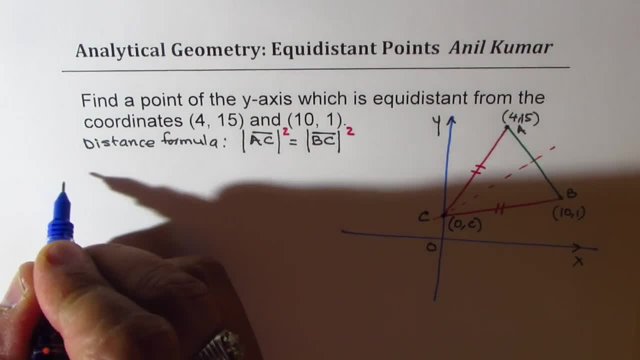 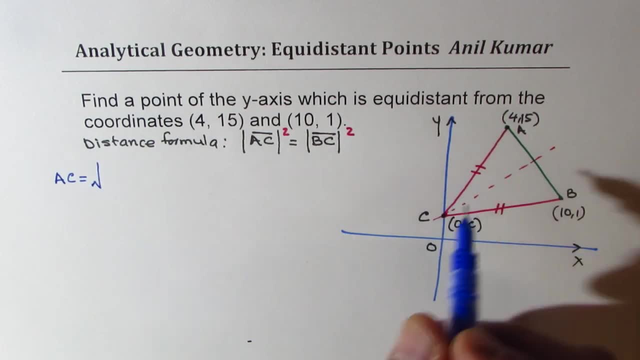 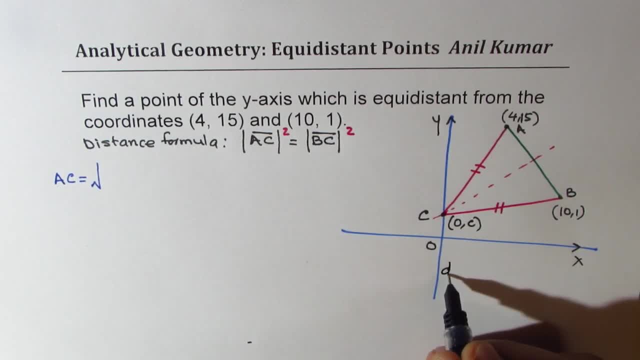 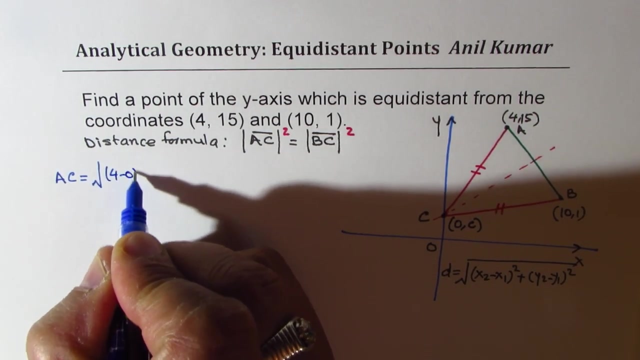 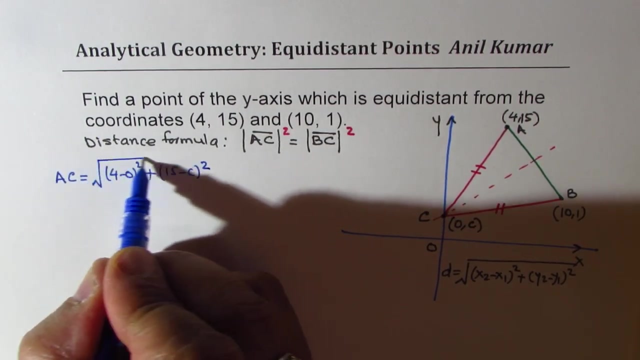 Let me write formula here. So the distance formula is: distance is equal to X2 minus X1, whole square, plus Y2 minus Y1 whole square square. That's the distance formula. So distance between a and c will be 4 minus 0, which is- let me write: 4 minus 0 whole square, plus 15 minus c whole square, That is a c. 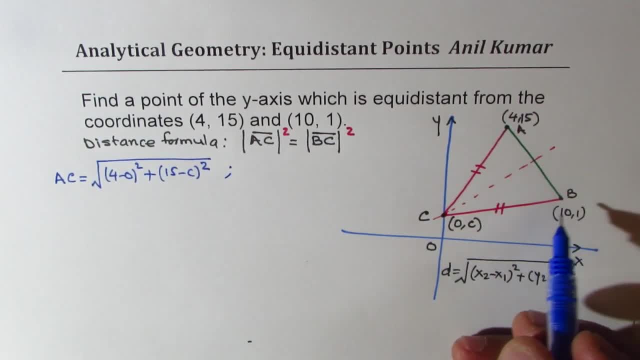 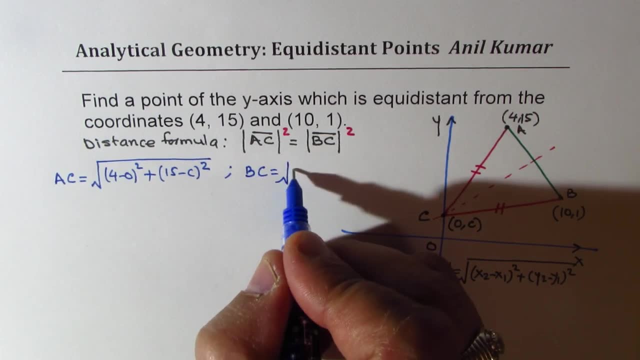 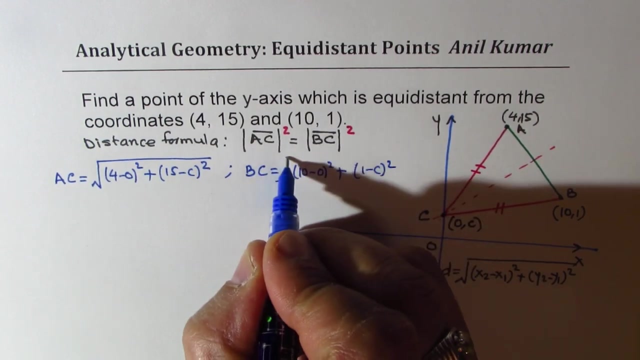 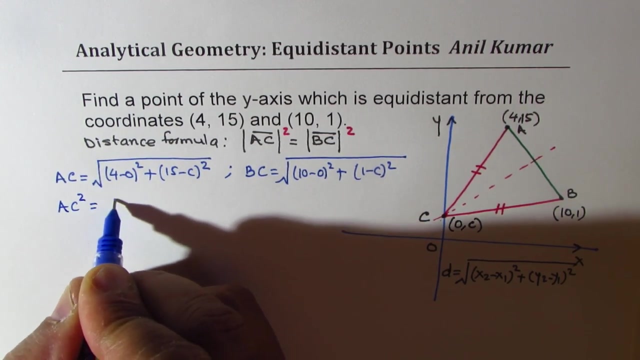 Now what is b c? b c will be equal to 10 minus 0 whole square, plus 1 minus c whole square. Now, if that is the case, we also know that their squares will also be equal, right, So equating their squares. 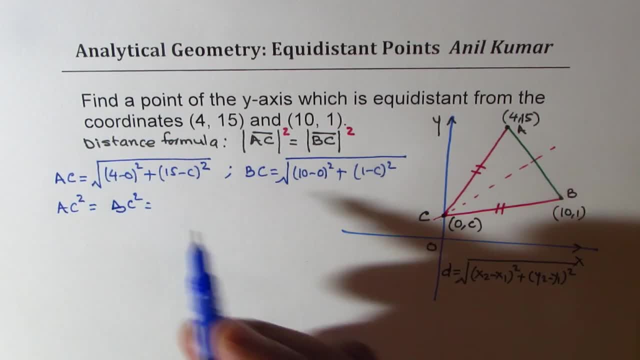 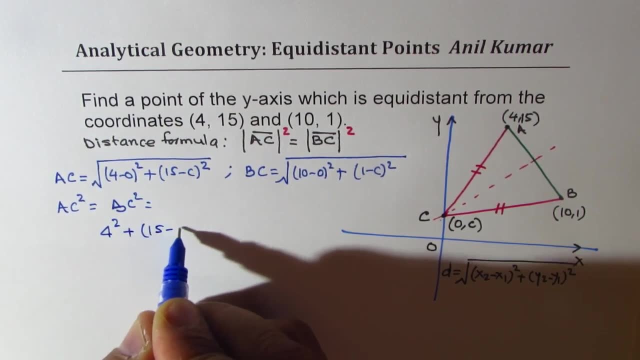 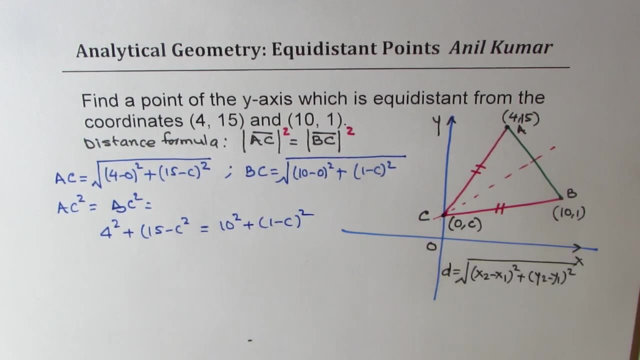 what is b? c? What do we get? We get this. This is 4 square, right. So we have 4 square plus 15 minus c. whole square should be equal to 10 square plus 1 minus c whole square. 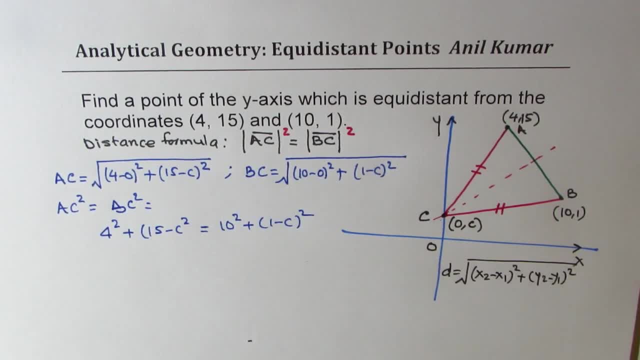 No problems, We just squared this right. So if you square, I mean, then the square root vanishes, You get a positive value. So we get this equation. Now only one variable is there to be solved, which is c. 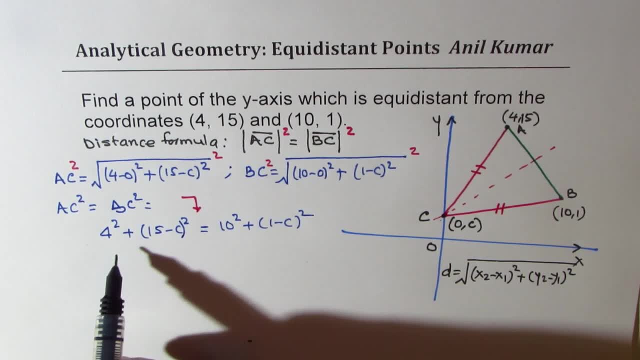 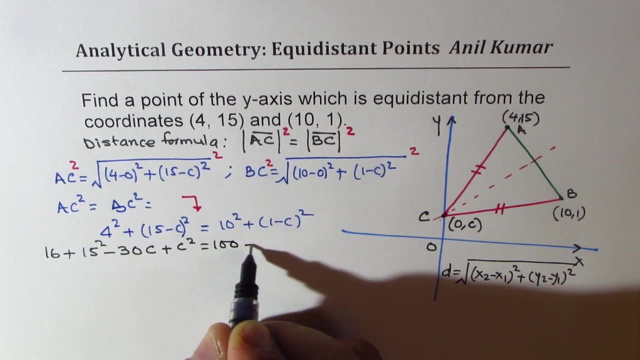 So let's expand and solve it. So what we get here is 16 plus 15 square. let me write 15 square minus 2ab, which is 30c plus c. square should be equal to 100 plus 1 minus 2c. 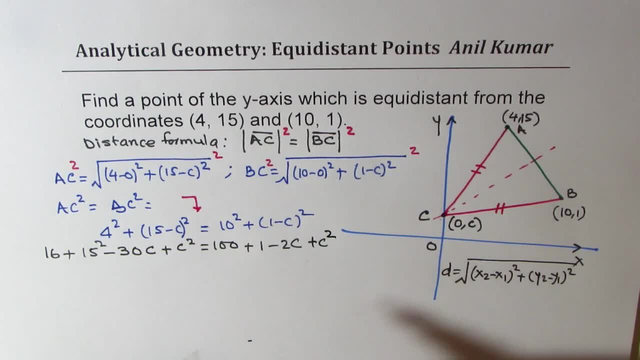 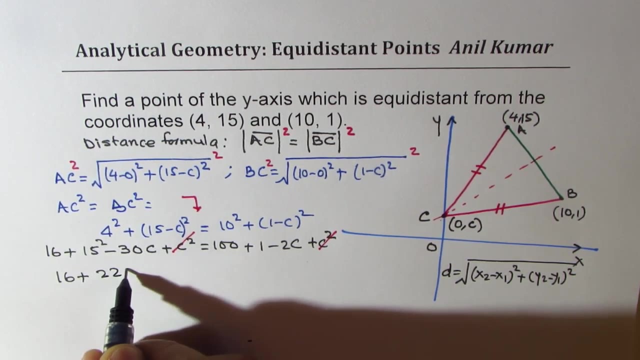 Okay Now from this equation, the c square, c square cancels. we can bring c on one side, numbers on the other. so we have 16 plus 15. square is 225, we'll bring 100 this side. so minus 100, minus 1 is equal to bringing 30 to the other side, gives us plus 30c. we have minus 2c here. 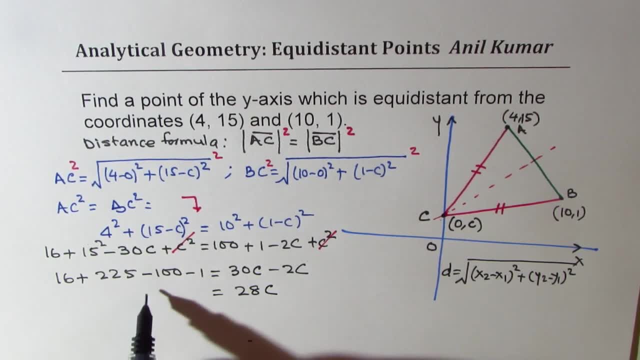 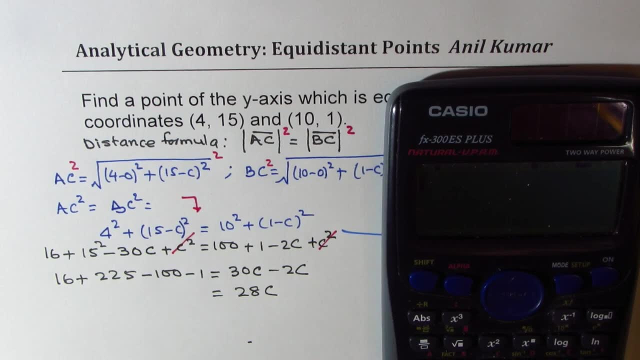 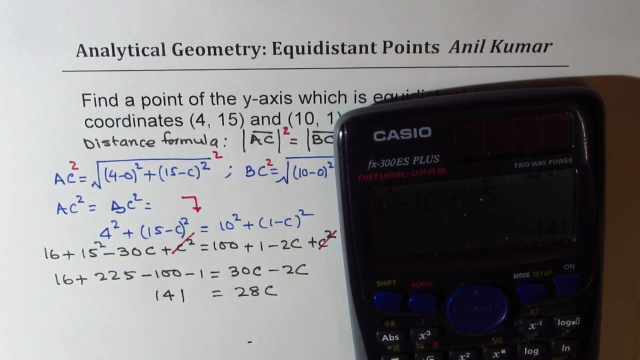 So that is 28c, And we have here- let's use calculator- we need to divide by 28 to get our answer. so we have 16 minus 100 plus 225, which is 141, so we have 141 here. so we did 16 minus 100, and we have to take away 1 also, so it is 140,. take away 1.. 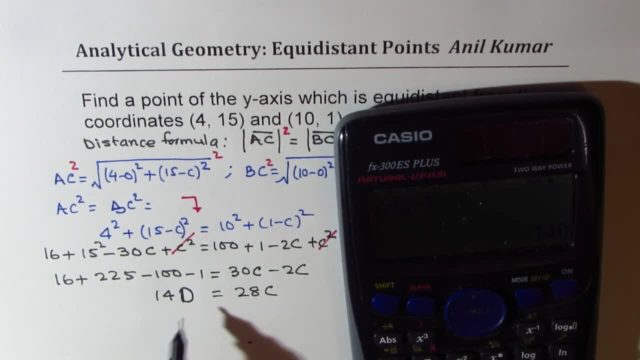 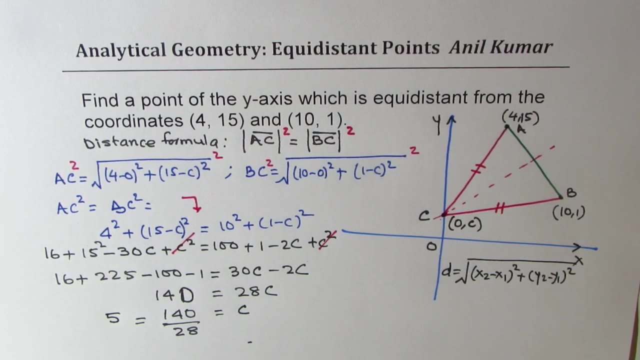 Okay, Okay, Okay, I forgot that. Okay, So it gives you 140.. Now, c is 140 divided by 28.. So let's divide this by 28.. We get the number 5.. So the y-intercept is, or, the point is 0, 5.. 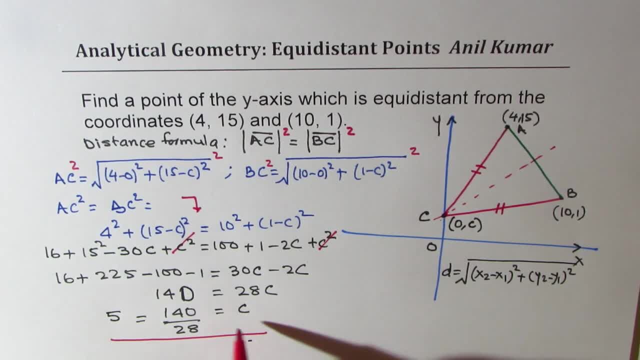 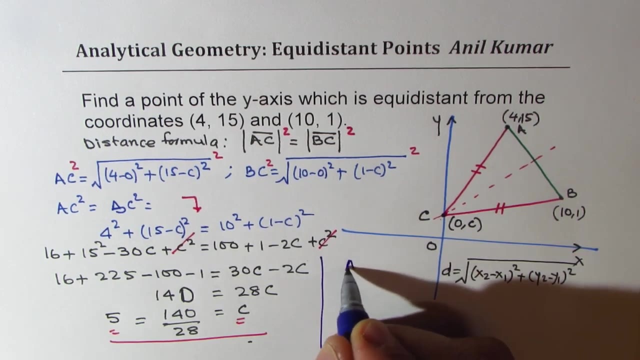 Do you see that part? So we get right our answer: c equals to 5.. So we can now write down that. But the point which is equidistant is indeed 0, 5.. So the answer is 0, 5 is same distance away.